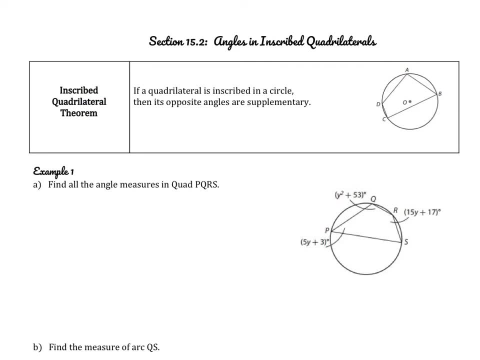 So the inscribed quadrilateral theorem states that if a quadrilateral is inscribed in a circle, then its opposite angles are supplementary. So remember, supplementary means that they add up to 180 degrees. So from this figure to the right, we could say angle A plus angle C. 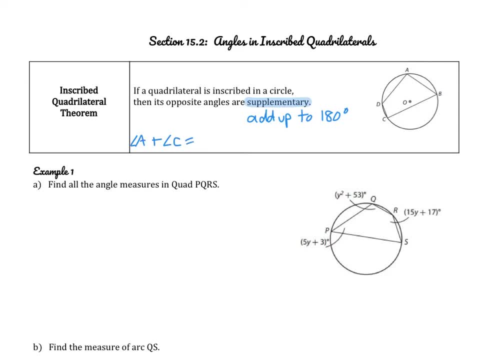 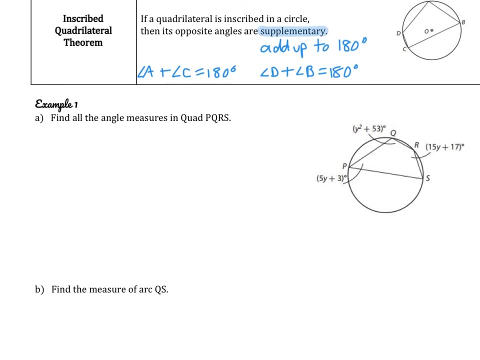 equals 180, and we could also make the equation that angle D plus angle B equals 180.. All right, so let's see if we can use the inscribed quadrilateral theorem to help us with these examples. So first we're asked to find all the angle measures in quadrilateral PQRS. 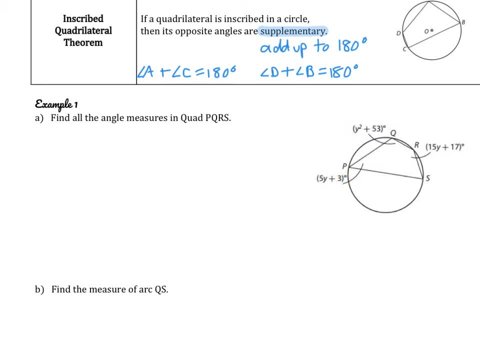 So, to start, we are going to need to first figure out what that y value is. and again, we know that the opposite angles are supplementary. So we know that angle P and angle R are supplementary. So we can make the statement: angle P plus angle R equals 180 degrees. and then we 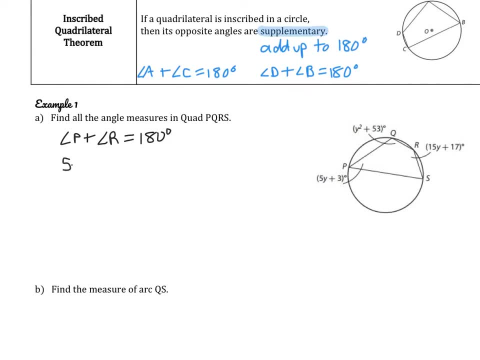 can substitute their values and we can solve for y. So 5y plus 3 plus 15y plus 17 equals 180.. Let's combine like terms. So here we get: 20y plus 20 equals 180.. 20y equals 160.. So y equals 8.. 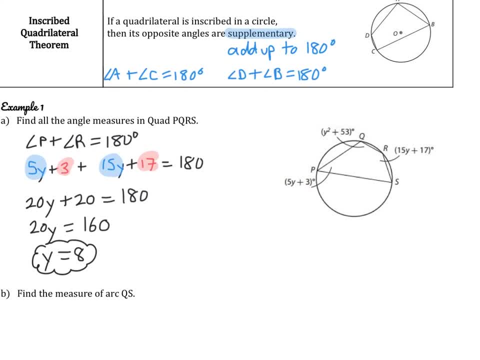 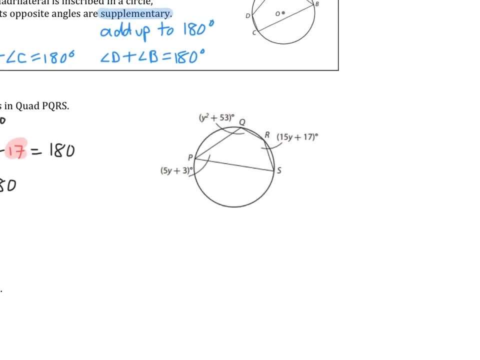 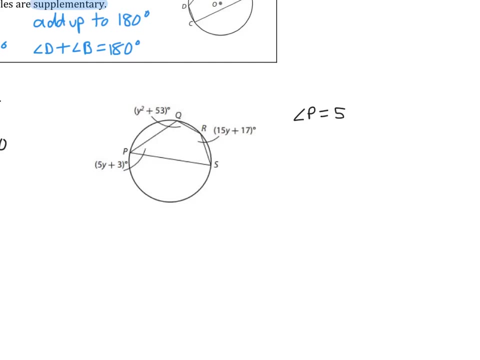 So now we can use that to help us find what the actual measure measurements are. So we're going to need to substitute them into each movement, into each你說 angle. we'll substitute y equals 8 to find the value. So let's start with angle P, We'll do 5. 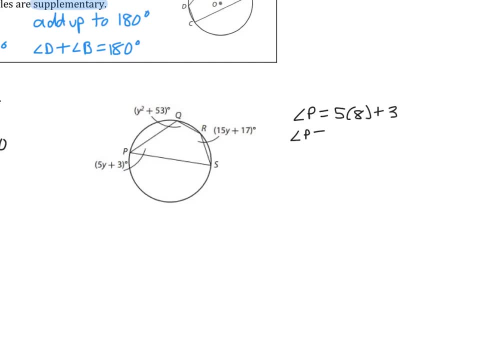 times 8 plus 3.. So angle P is 43 degrees. Angle R is going to be 15 times 8 plus 17.. So angle R equals 137 degrees, which checks out because, remember, these two angles should be supplementary and they do add up to 180.. Let's do angle Q, So it's going to be 8 squared plus 53.. 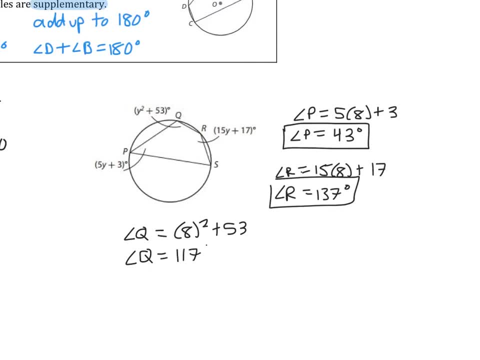 So angle Q equals 117 degrees. And then, to find angle X, we have two options. We could either do 360 minus angle P, minus angle R, minus angle Q, because, remember, the angles within a quadrilateral should add up to 360.. Or again, we know. 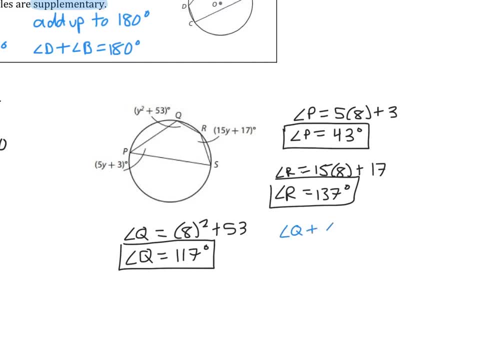 that angle Q and angle S are supplementary because they are opposite each other, so they should add up to 180.. So we can substitute what we know for angle Q And we could solve for angle S. So angle S equals 63 degrees. 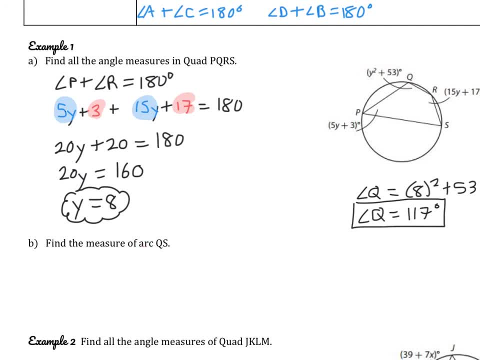 Okay, now, using the same figure, now we're going to find the measure of arc QS. Okay, so if we're trying to find the measurement of this arc, notice that the measurement of that arc is going to be 63 degrees. So if we're trying to find the measurement of this arc, 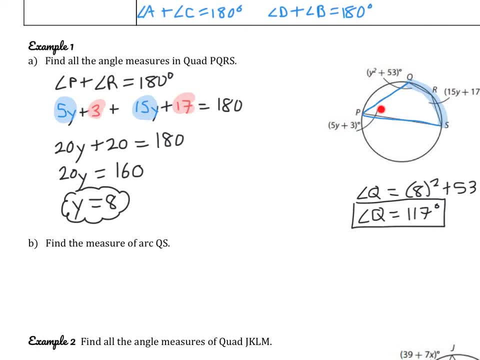 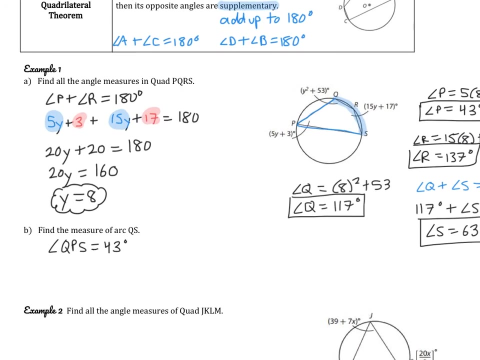 is simply going to be double the measurement of this angle, because this is an inscribed angle And we know that angle QPS is equal to 43 degrees. We just found that out in the first part. So, again, the arc is simply going to be double that. So the measure of arc QS is 86 degrees. 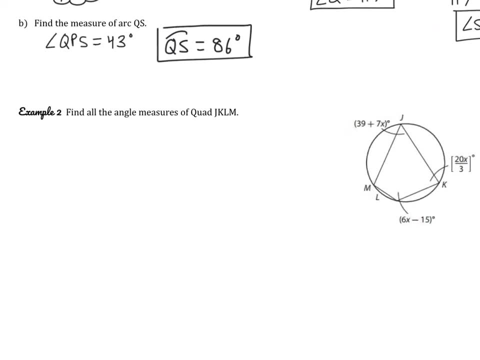 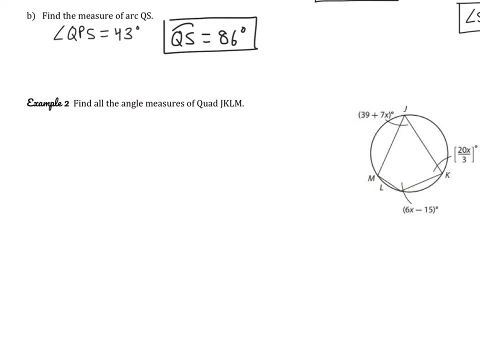 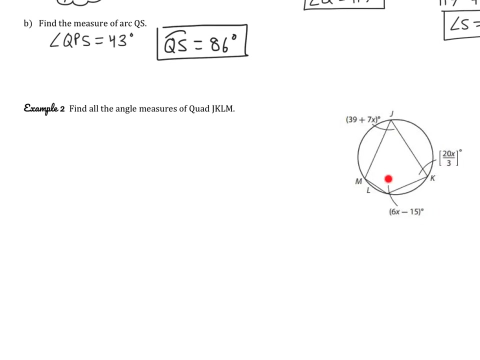 All right, let's look down here at example two. So this one says: find the angles, measures of quadrilateral JKLM. So same idea we're first in need to solve for axe, and we can do that by creating an equation using our supplementary angles. So let's use angles J and L. 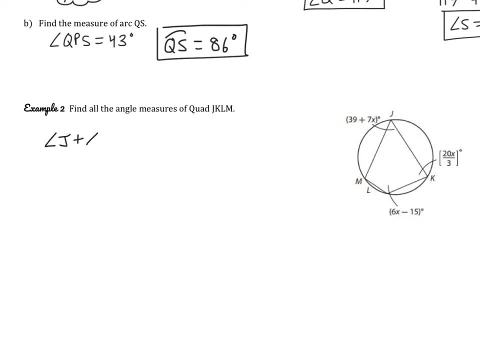 So we know that angle J plus angle L should equal 180, because they are opposite it and are therefore supplementary. So 39 plus 7x plus 6x minus 15 equals 180. So if we combine like terms, we get: 13x plus 24 equals 180.. So 13x equals 156.. And if we divide, 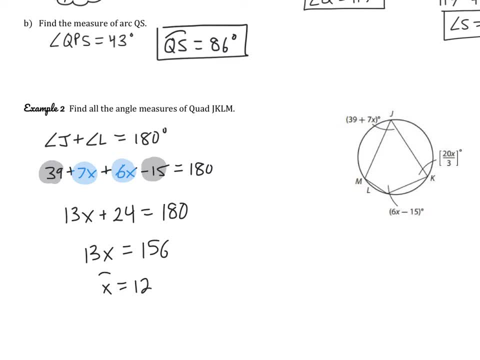 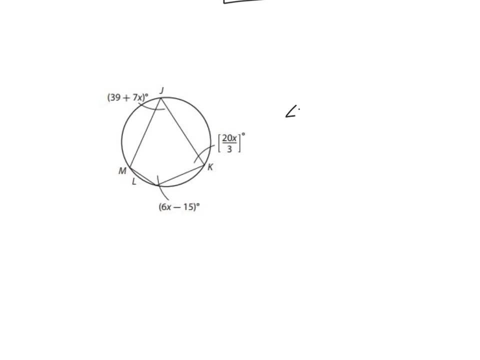 both sides by 13, we get x equals 12.. So again we can then go and substitute x to find all of our terms Angles. So angle J is going to be 39 plus 7 times 12.. So angle J is going to be 123. 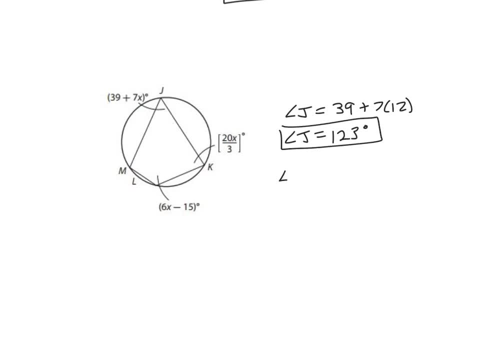 degrees, Angle L is going to be 6 times 12 minus 15.. Angle L is going to be 57 degrees, And again, this checks out, because these two angles should add up to 180, and they do. Let's find angle K. So angle K is going to be 20 times 12 divided by 3.. So we 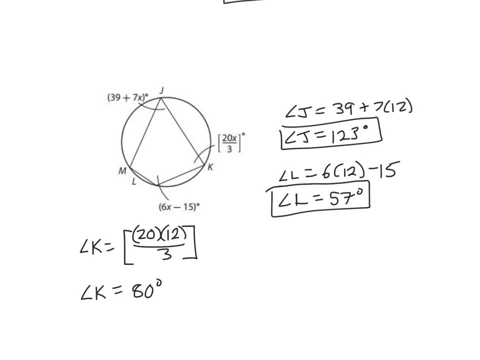 get, angle K is 80 degrees, And then we see that angle M is opposite angle K. So these two angles should be supplementary. So we can say angle M plus angle K equals 180 degrees. We know that angle K is 80. So 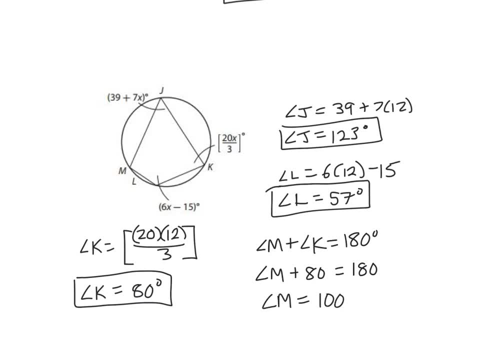 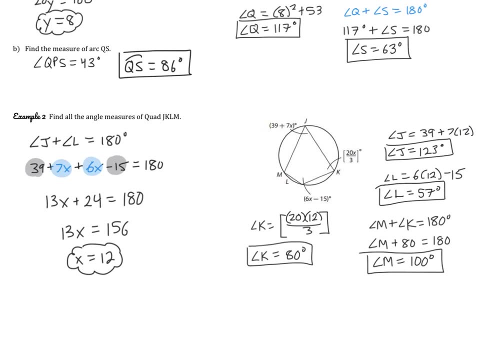 therefore, angle M must be 100 degrees, And that's all there is to it. Alright, that is all for today's video. Thank you so much for watching, and I'll see you in the next video. Bye, Thank you so much for watching.